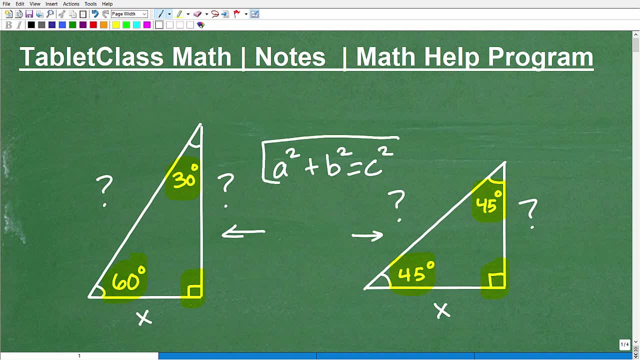 However, oftentimes you cannot use this theorem. It's not enough, given the information for these particular problems. You might need some trigonometry. But you know, if you don't, if we can't use a Pythagorean theorem, if we can't use trigonometry, then we can use these special properties of the 30,, 60,, 90 and 45,, 45, 90 degree triangle. 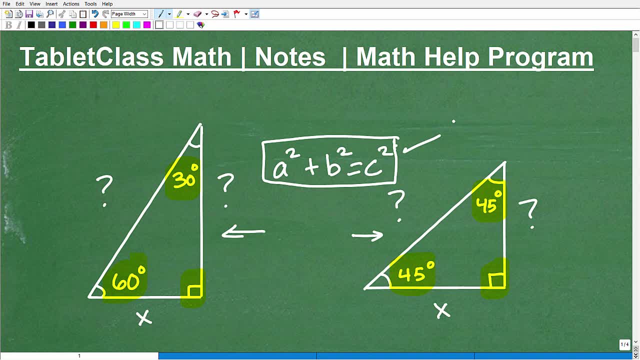 So we're going to get into this in just one second. It's very, very important for those of you That are you know whether you're taking geometry or not. you just got to know this, Okay, so we're going to get into this again in just one second. But first let me quickly introduce myself. My name is John. I'm the founder of Tab of Class Math. 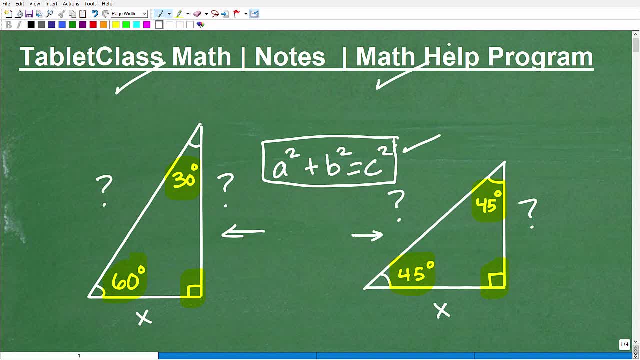 I'm also a middle and high school math teacher And over several years I've constructed what I like to believe is one of the best online math help programs there is. Of course, I'll let you be the judge of that. You can find a link to my math help program in the description of this video. 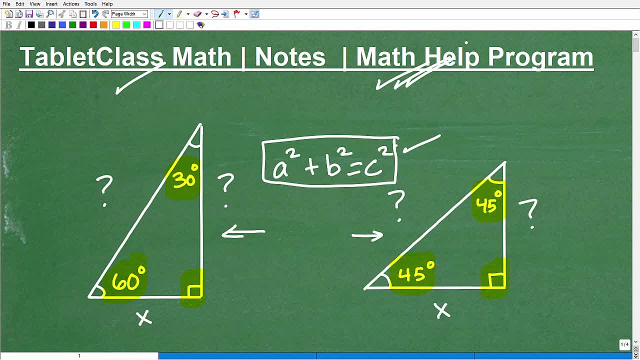 But basically I have 100 plus different math courses. all the big courses: pre-algebra, algebra 1, geometry algebra 2, college algebra. I'm going to be launching a pre-calculus here soon, But I have a ton of other type of courses, test preparation courses. 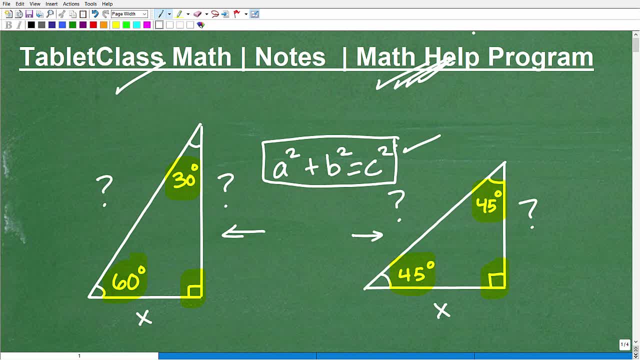 So if you're studying for the GED, SAT, ACT, GRE, GMAT, ACCUPLACER, ALEKS, teacher certification, nursing, entrance, it doesn't make a difference. There's a ton of different tests that are very, very important for people's goals. 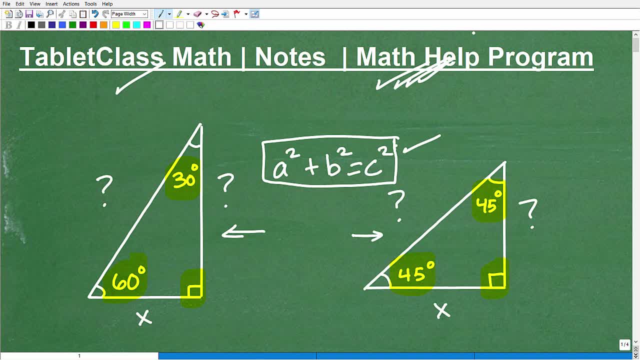 Okay, whether it's you know, to get into a particular program, get a certification. So a lot of people study mathematics, have to study math Okay Because that's on their you know- particular exam they're facing. So I recognize that I have very comprehensive, excellent test preparation math courses. 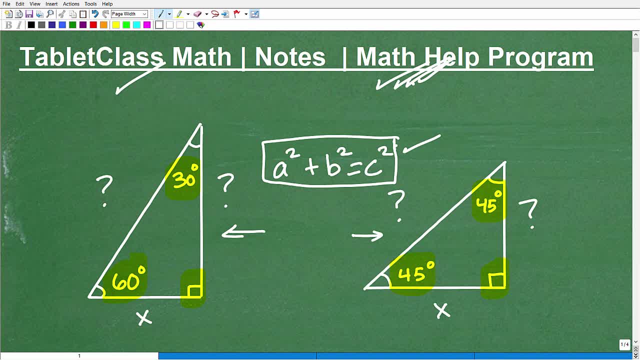 So you can check out my full catalog. Just go on to my website. Hopefully I have what you are studying If I don't, drop me a line in my contact form and I'll help you out the best. I can Also deal out with independent learners like homeschoolers. 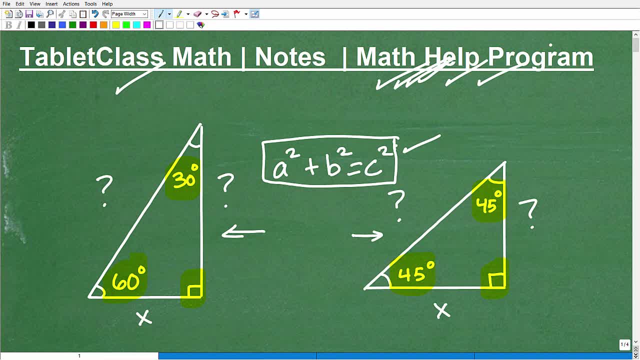 I have a great homeschool learning system And then, obviously, if you're just struggling in math class, I can help you out. But for those of you you know that are struggling in any math- mathematics or studying math- you just need to know how important it is to take notes. 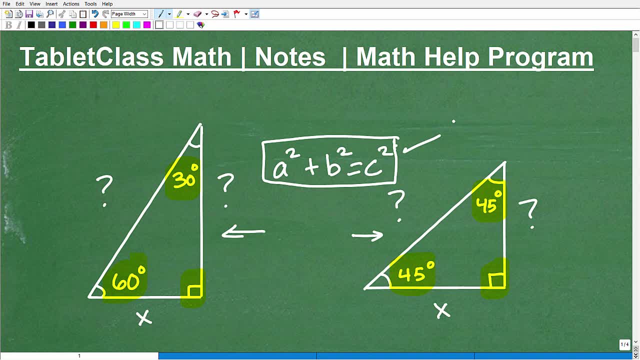 So we're going to get into this in just one second. It's very, very important for those of you That are you know whether you're taking geometry or not. you just got to know this, Okay, so we're going to get into this again in just one second. But first let me quickly introduce myself. My name is John. I'm the founder of Tab of Class Math. 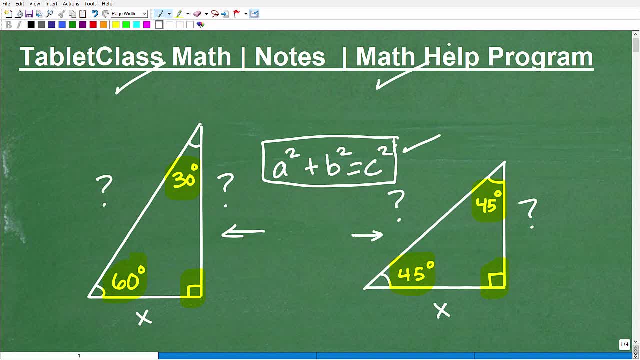 I'm also a middle and high school math teacher And over several years I've constructed what I like to believe is one of the best online math help programs there is. Of course, I'll let you be the judge of that. You can find a link to my math help program in the description of this video. 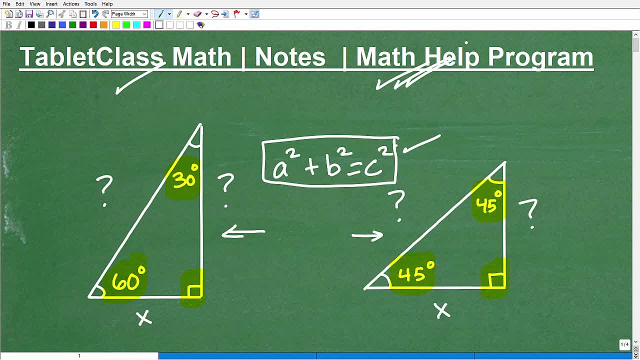 But basically I have 100 plus different math courses. all the big courses: pre-algebra, algebra 1, geometry algebra 2, college algebra. I'm going to be launching a pre-calculus here soon, But I have a ton of other type of courses, test preparation courses. 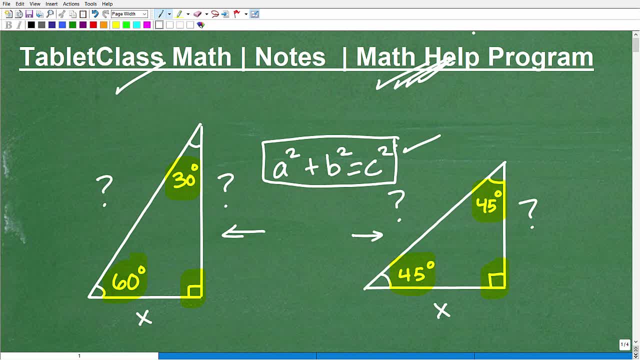 So if you're studying for the GED, SAT, ACT, GRE, GMAT, ACCUPLACER, ALEKS, teacher certification, nursing, entrance, it doesn't make a difference. There's a ton of different tests that are very, very important for people's goals. 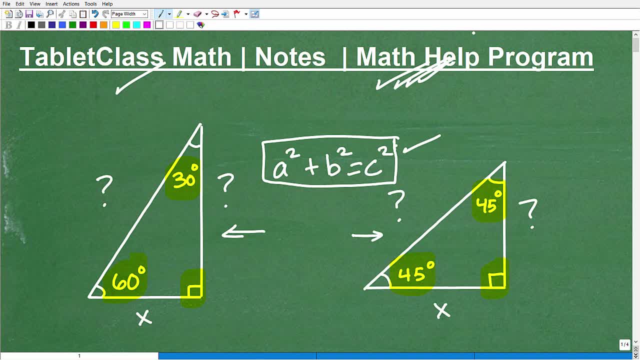 Okay, whether it's you know, to get into a particular program, get a certification. So a lot of people study mathematics, have to study math Okay Because that's on their you know- particular exam they're facing. So I recognize that I have very comprehensive, excellent test preparation math courses. 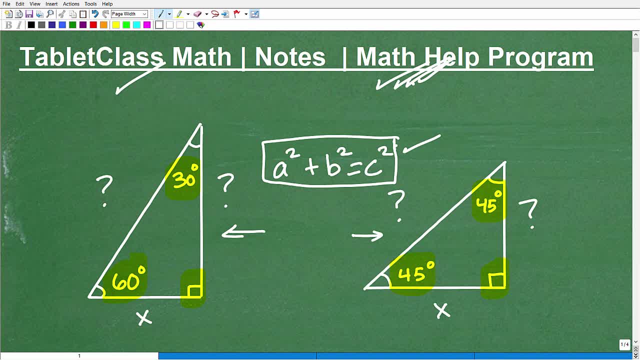 So you can check out my full catalog. Just go on to my website. Hopefully I have what you are studying If I don't, drop me a line in my contact form and I'll help you out the best. I can Also deal out with independent learners like homeschoolers. 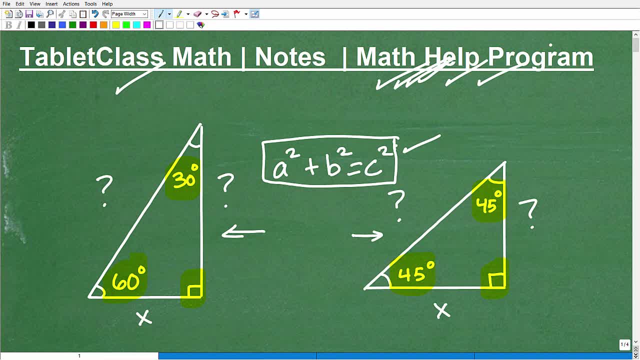 I have a great homeschool learning system And then, obviously, if you're just struggling in math class, I can help you out. But for those of you you know that are struggling in any math- mathematics or studying math- you just need to know how important it is to take notes. 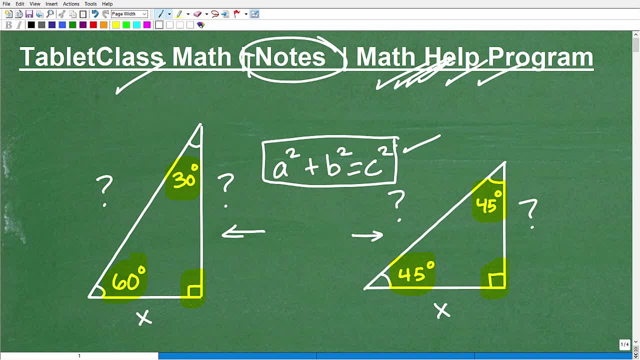 I call this my golden rule of mathematics. Over decades of teaching math, one thing is apparent to me: Those students who take great math notes almost always end up with great math grades, And the reverse is true: Those students who just not into taking notes, rather do other stuff or just distracted. you know, I get it. 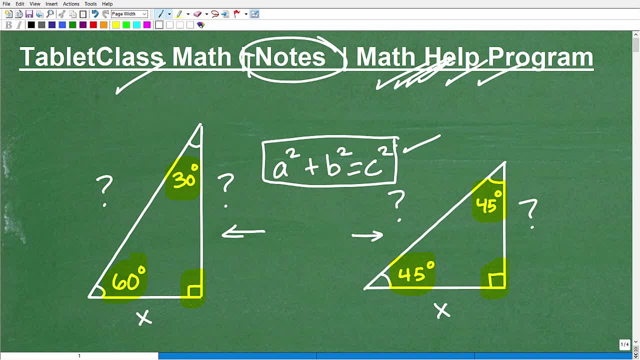 I call this my golden rule of mathematics. Over decades of teaching math, one thing is apparent to me: Those students who take great math notes almost always end up with great math grades, And the reverse is true: Those students who just not into taking notes, rather do other stuff or just distracted. you know, I get it. 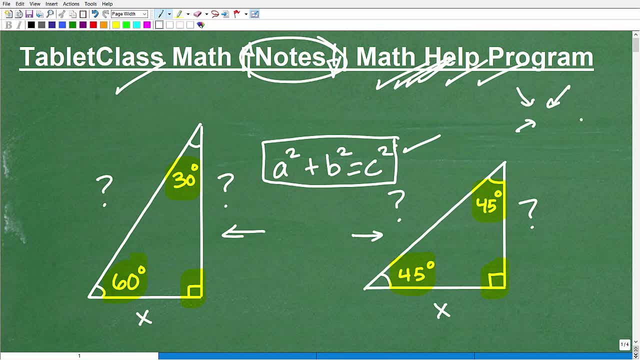 You know there's so much information coming at us, you know, all the time, And having our cell phones even makes it that much worse, right? So the only way you're going to remain focused on the instruction that's coming in your way from your teacher is to be engaged in an activity that forces you to stay focused and that's note taking, okay. 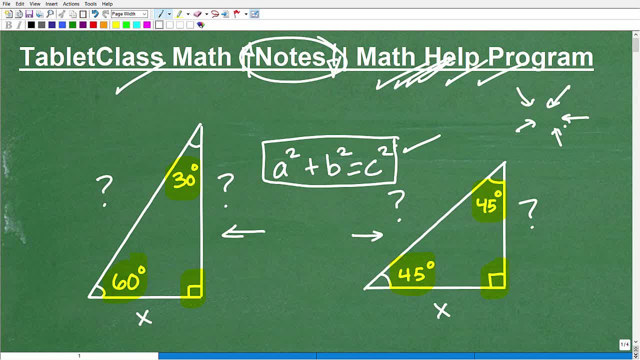 Just believe me on this one. I've been doing this for a long, long time. If you improve your notes, everything else is going to get better for you in terms of mathematics. But you know as you're doing that it is. you know something that requires effort and is a skill, or slash art form, if you will. 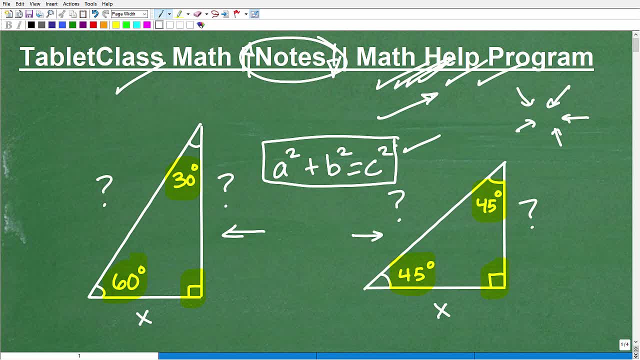 To take great math notes, And it's something you have to practice. Over time you'll get better at it, But as you are getting better at it, you still need something to study from. So I offer detailed, comprehensive math notes to include pre-algebra, algebra 1,, geometry, algebra 2, and trigonometry. 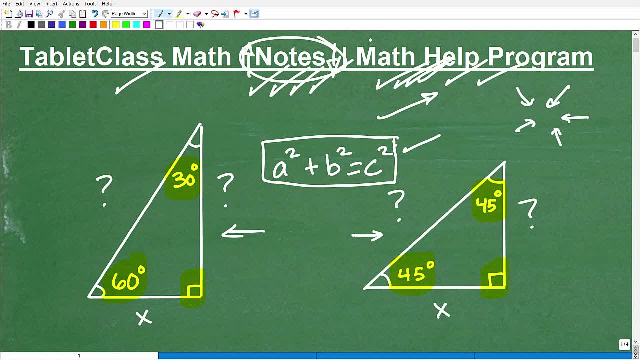 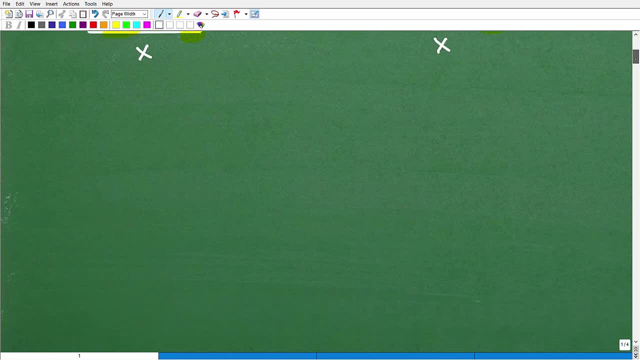 Okay, so let's get into this, these two triangles, And we classify these as special right triangles. okay, So let's talk about special right triangles, But before we do that, let's just look at any old triangle. This, any old right triangle. 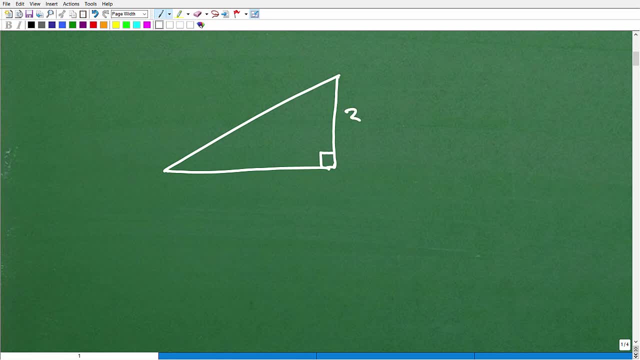 So let's say I have a right triangle and this was 3, and this was 4. And I said: find the length of the hypotenuse Okay. now, in this particular situation, we have this length and this length. 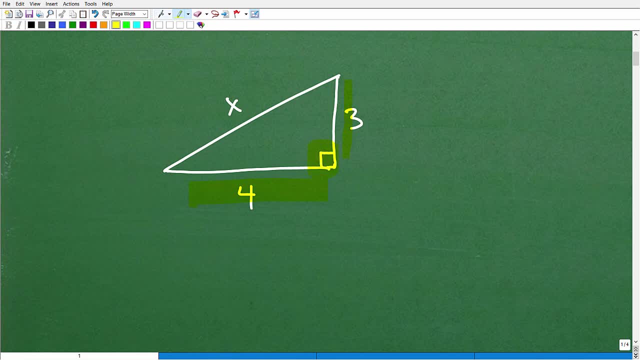 So we have two of the three missing sides. We know it's the right triangle, So I could simply go ahead and use the Pythagorean Theorem. okay, And we would go ahead. This would be: 3 squared plus 4 squared is equal to C squared. 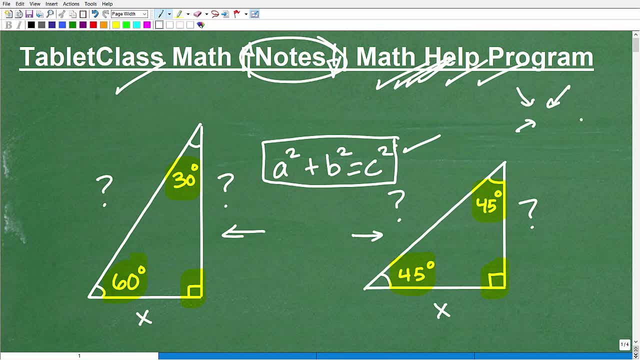 You know there's so much information coming at us, you know, all the time, And having our cell phones even makes it that much worse, right? So the only way you're going to remain focused on the instruction that's coming in your way from your teacher is to be engaged in an activity that forces you to stay focused and that's note taking, okay. 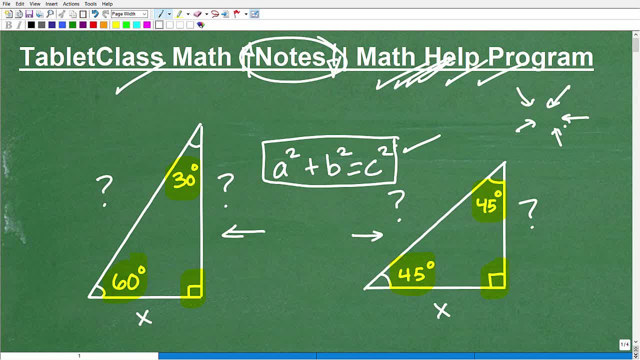 Just believe me on this one. I've been doing this for a long, long time. If you improve your notes, everything else is going to get better for you in terms of mathematics. But you know as you're doing that it is. you know something that requires effort and is a skill, or slash art form, if you will. 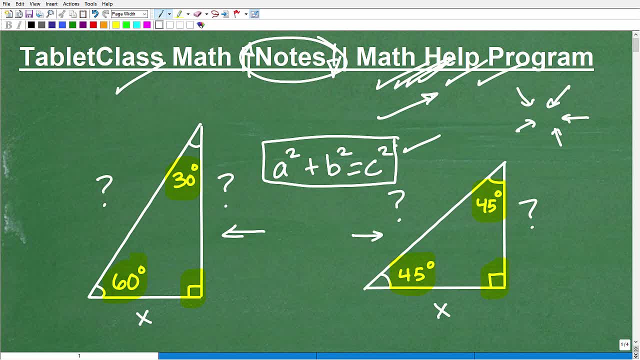 To take great math notes, And it's something you have to practice. Over time you'll get better at it, But as you are getting better at it, you still need something to study from. So I offer detailed, comprehensive math notes to include pre-algebra, algebra 1,, geometry, algebra 2, and trigonometry. 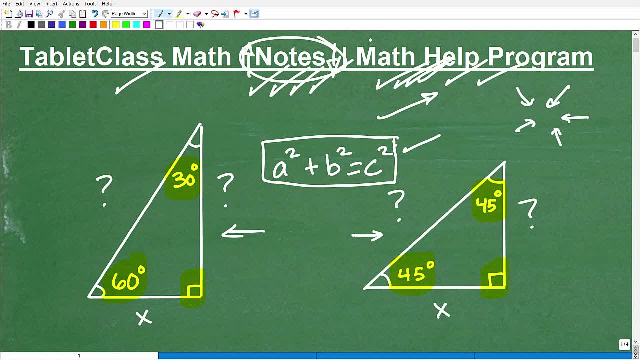 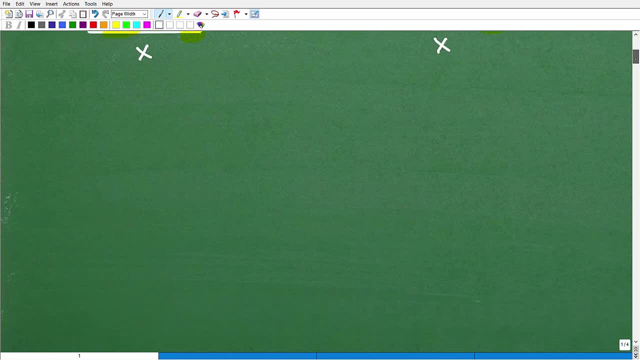 Okay, so let's get into this, these two triangles, And we classify these as special right triangles. okay, So let's talk about special right triangles, But before we do that, let's just look at any old triangle. This, any old right triangle. 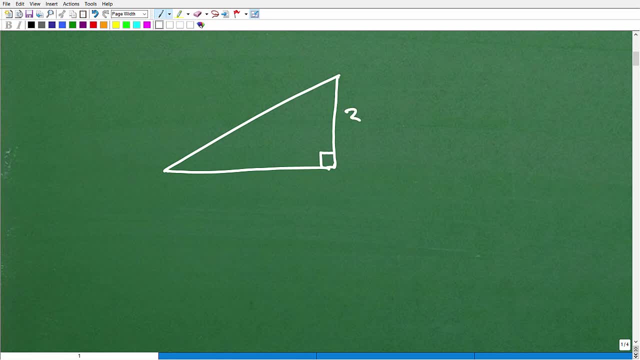 So let's say I have a right triangle and this was 3, and this was 4. And I said: find the length of the hypotenuse Okay. now, in this particular situation, we have this length and this length. 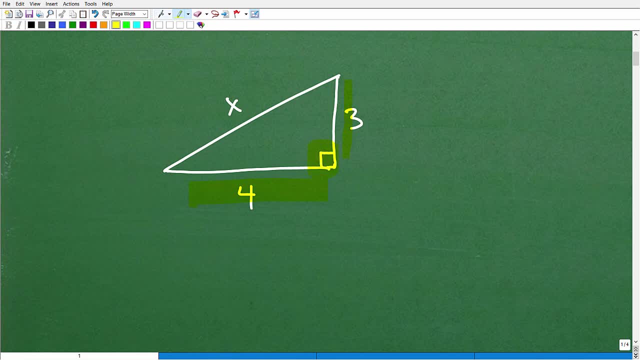 So we have two of the three missing sides. We know it's the right triangle, So I could simply go ahead and use the Pythagorean Theorem. okay, And we would go ahead. This would be: 3 squared plus 4 squared is equal to C squared. 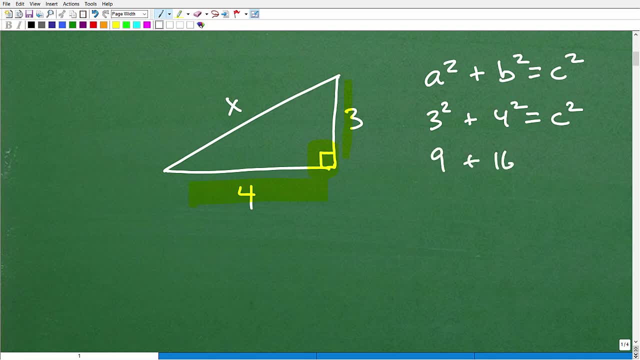 And then we would end up with 9 plus 16 is equal to C squared. C squared is this side. And, by the way, this is just a quick review on the Pythagorean Theorem. If you really need to, you know review this or learn this, just check out. I have tons of videos on this in my geometry playlist. 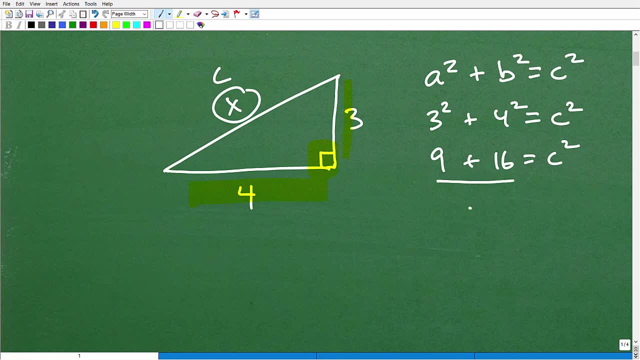 You can learn all about the Pythagorean Theorem there, But we have 9 plus 16 is 25 is equal to C squared. I take the square root of both sides And C is equal to 5.. So the missing length of this particular triangle is 5.. 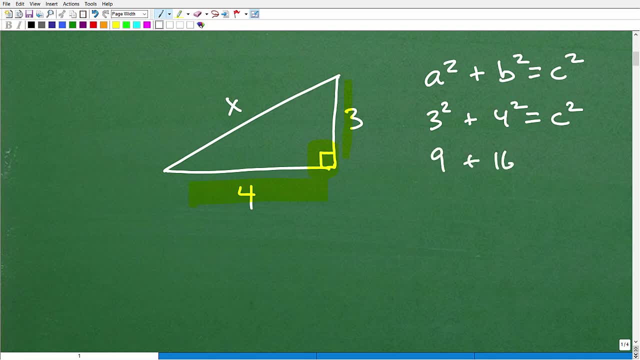 And then we would end up with 9 plus 16 is equal to C squared. C squared is this side. And, by the way, this is just a quick review on the Pythagorean Theorem. If you really need to, you know review this or learn this, just check out. I have tons of videos on this in my geometry playlist. 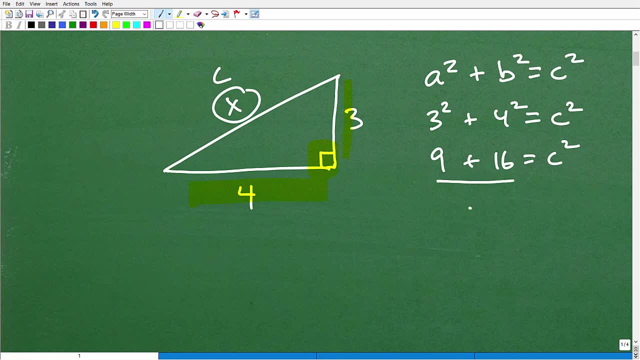 You can learn all about the Pythagorean Theorem there, But we have 9 plus 16 is 25 is equal to C squared. I take the square root of both sides And C is equal to 5.. So the missing length of this particular triangle is 5.. 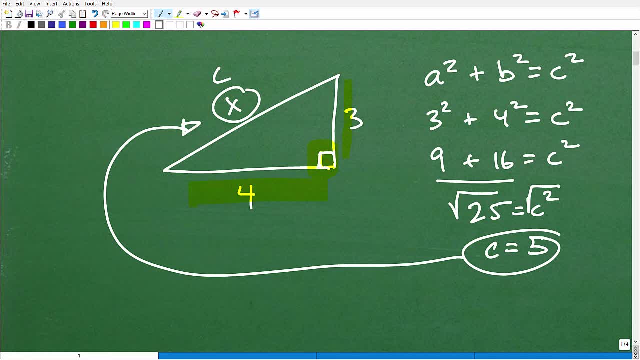 So pretty straightforward. So, when we have a right triangle, you want to be thinking Pythagorean Theorem. okay, However, what happens if I don't have two lengths? okay, So let's say it's this situation, right? 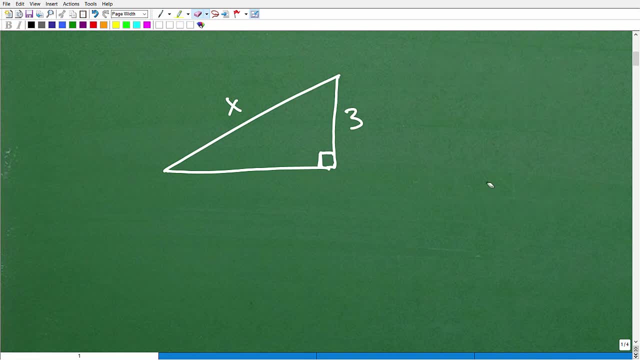 And I'm like, hmm, okay, well, what's going on here? Well, here you're stuck, You can't do anything, okay, because we don't have enough information. I just have this side and this length, okay. 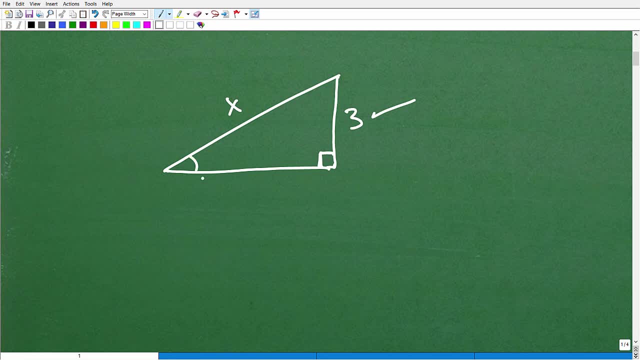 I need some additional information Now. if you had, let's say, this angle, let's say this angle was 20 degrees, then you could use trigonometry- okay, Some basic trigonometry that involves the sine, cosine and tangent, to figure this out. okay. 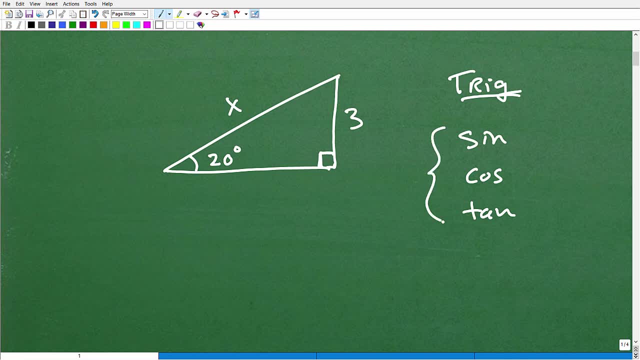 Now this is again involves trigonometric ratios and might be beyond the scope of what you're studying Right now, but this is what would be required. okay, You would need trigonometry, okay. However, there are triangles where we don't have to use trigonometry and, of course, we can't use the Pythagorean Theorem. 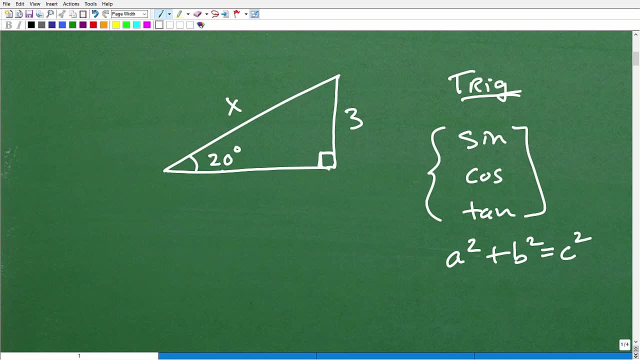 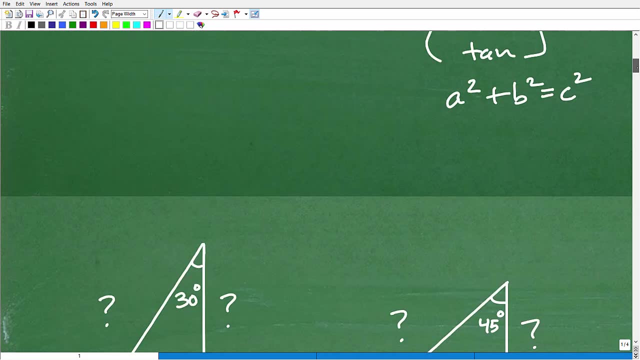 because we don't have two sides here or we just have an angle. So those situations are these special right triangles and you need to know these rules, okay? So, when you encounter a 30-60-90 or a 45-45-90,. 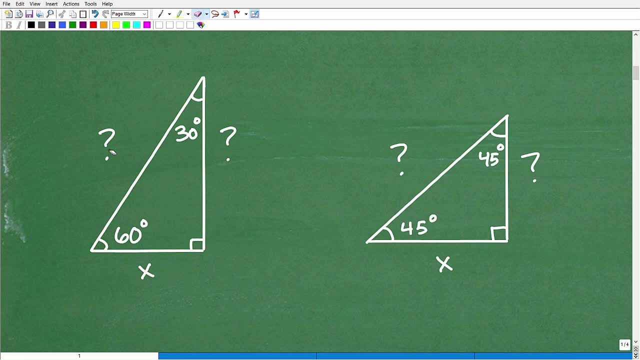 okay, you need to know these rules, So let's go ahead and take a look at the 30-60-90 first. All right, so let's say this side here is x, Let's call it x equals 2, and I want to find these remaining two sides right. 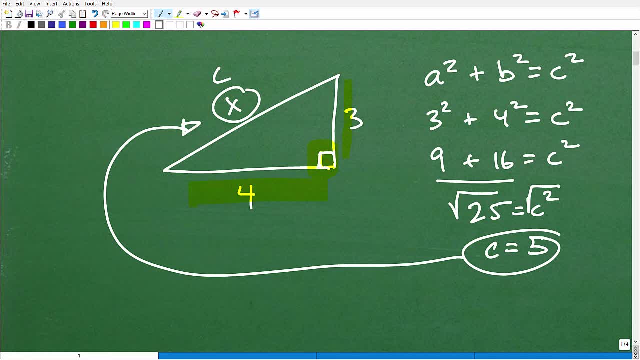 So pretty straightforward. So, when we have a right triangle, you want to be thinking Pythagorean Theorem. okay, However, what happens if I don't have two lengths? okay, So let's say it's this situation, right? 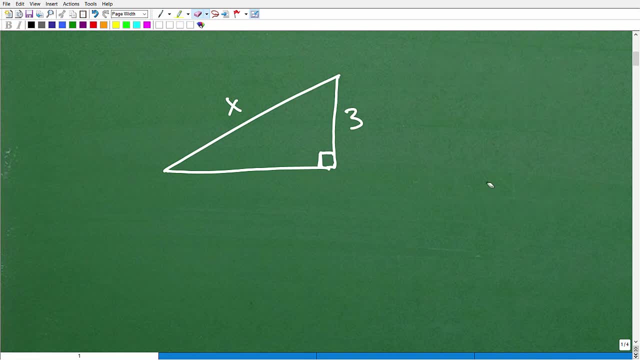 And I'm like, hmm, okay, well, what's going on here? Well, here you're stuck, You can't do anything, okay, because we don't have enough information. I just have this side and this length, okay. 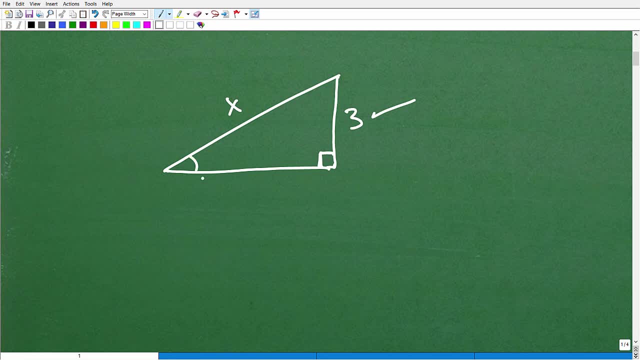 I need some additional information Now. if you had, let's say, this angle, let's say this angle was 20 degrees, then you could use trigonometry- okay, Some basic trigonometry that involves the sine, cosine and tangent, to figure this out. okay. 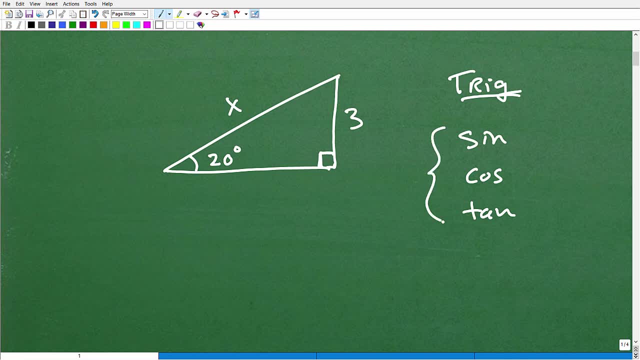 Now this is again involves trigonometric ratios and might be beyond the scope of what you're studying Right now, but this is what would be required. okay, You would need trigonometry, okay. However, there are triangles where we don't have to use trigonometry and, of course, we can't use the Pythagorean Theorem. 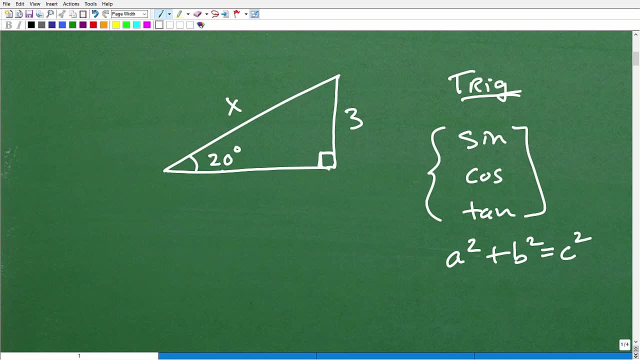 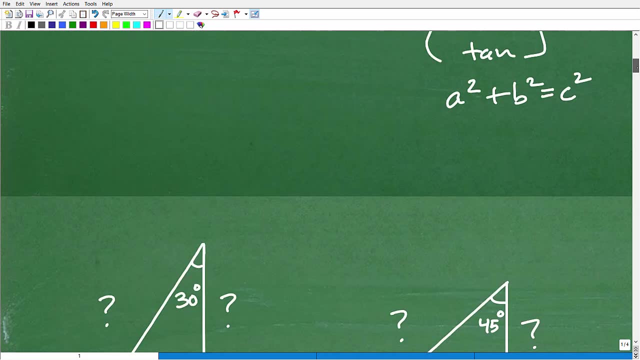 because we don't have two sides here or we just have an angle. So those situations are these special right triangles and you need to know these rules, okay? So, when you encounter a 30-60-90 or a 45-45-90,. 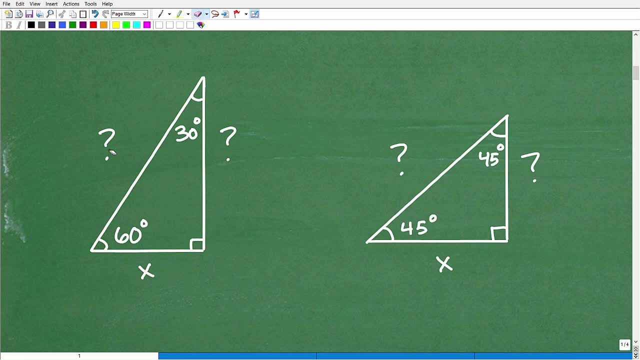 okay, you need to know these rules, So let's go ahead and take a look at the 30-60-90 first. All right, so let's say this side here is x, Let's call it x equals 2, and I want to find these remaining two sides right. 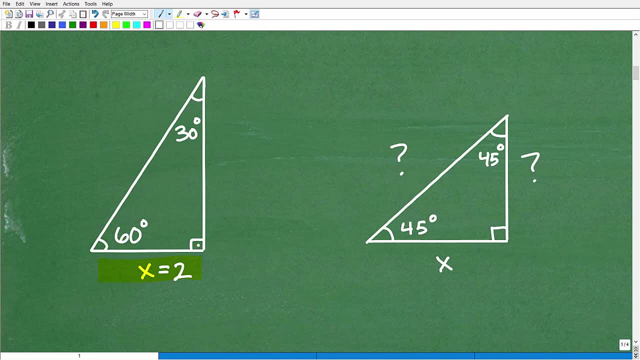 Well, again, I have one side, I have some angles, I know it's a right triangle, so it's not enough information for me to use the Pythagorean Theorem. okay, I can't do that, all right, So I would need. 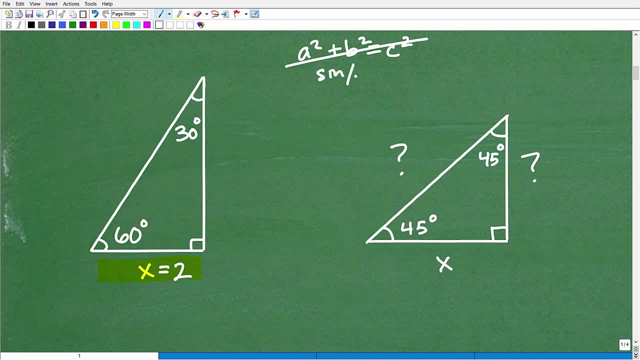 I need some trigonometry, yeah, but I don't want to be using sine, cosine and tangent again. So what we have is some basic, like a basic kind of rule here. all right, And when you have a 30-60-90, the sides of the triangle, of a 30-60-90 triangle, 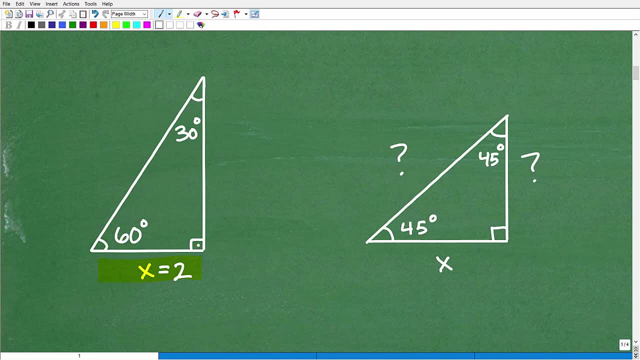 Well, again, I have one side, I have some angles, I know it's a right triangle, so it's not enough information for me to use the Pythagorean Theorem. okay, I can't do that, all right, So I would need. 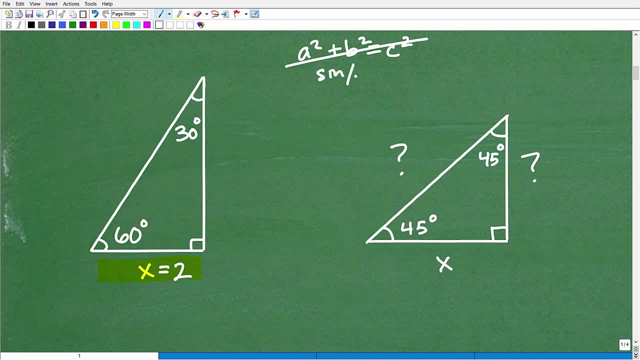 I need some trigonometry, yeah, but I don't want to be using sine, cosine and tangent again. So what we have is some basic, like a basic kind of rule here. all right, And when you have a 30-60-90, the sides of the triangle, of a 30-60-90 triangle, 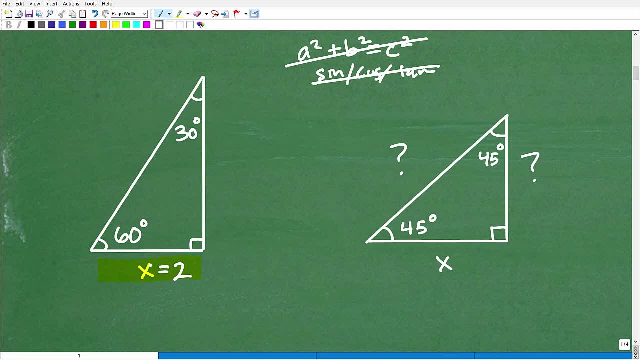 will always be in this proportion. So here is how it goes. all right, If this side is x, the hypotenuse will always be 2x. Okay, So it's double the smallest side. So this is the smallest side. 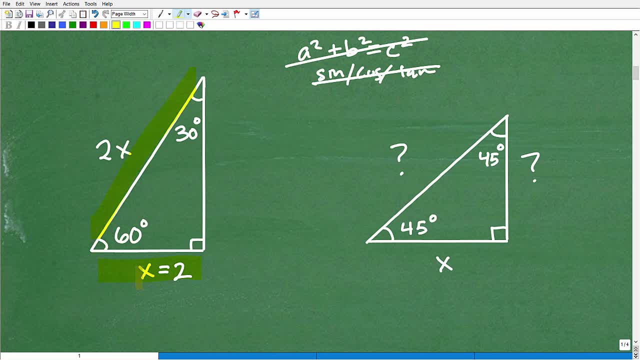 So this hypotenuse, the longest side will be double the smallest side. So that's really easy. That's 2 times 2, or 4.. So you're like, oh wow, that's super easy. 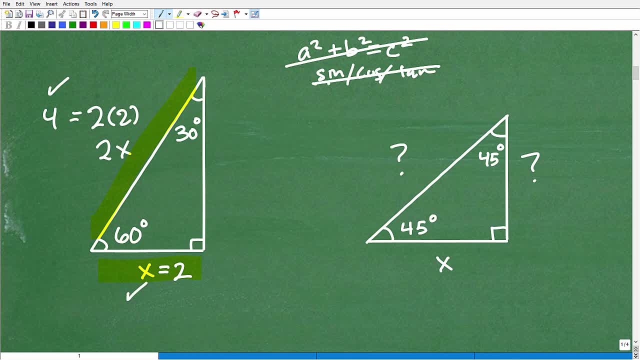 Now I have two lengths. Now, technically, you could now go and use the Pythagorean Theorem, but there's no need to do that. okay, This middle length. okay, not the shortest, not the longest, but this middle one. 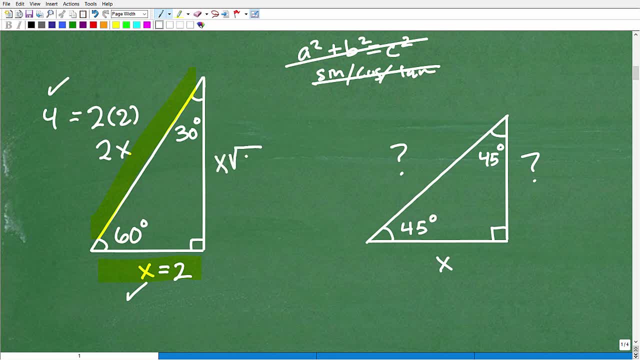 this one right here, This middle length right here is going to be x times the square root of 3.. So, whatever this value is here, this is 2 in this particular problem. So we just take that 2, and we multiply it by the square root of 3, and that's what this is. 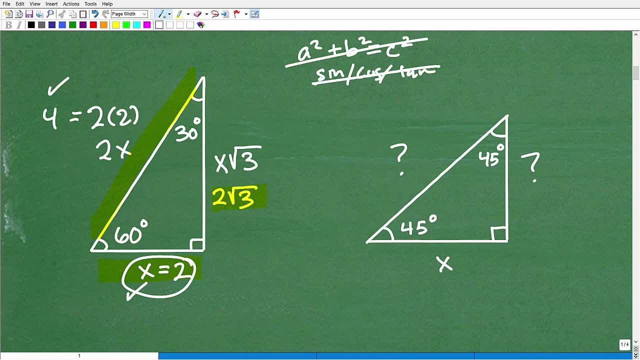 I mean easy as 1,, 2,, 3.. Now there's a lot more sophisticated kind of problems that you could do. I could give you this length of a 30-60-90, and then you would have to go and determine that. 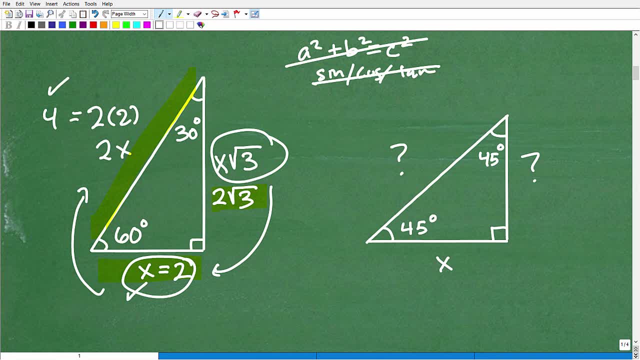 and then you could determine this, Or I could give you the hypotenuse. Actually, this is the hypotenuse. Actually, this is the hypotenuse. Let's do another quick problem here and let's see if you can remember all of this. 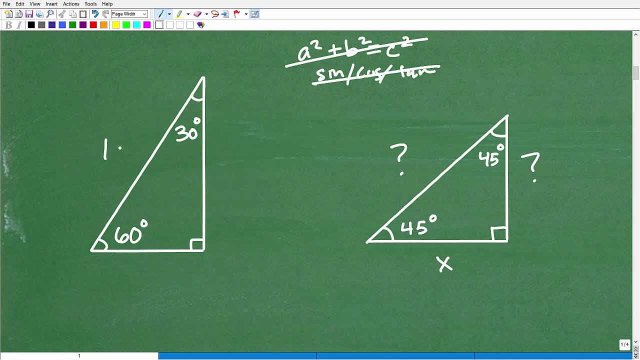 and we'll kind of reverse engineer the solution. So let's say this is 10,. all right, I give you this problem and I want you to know, I want you to go ahead and figure out what these sides are. So how could I approach that? 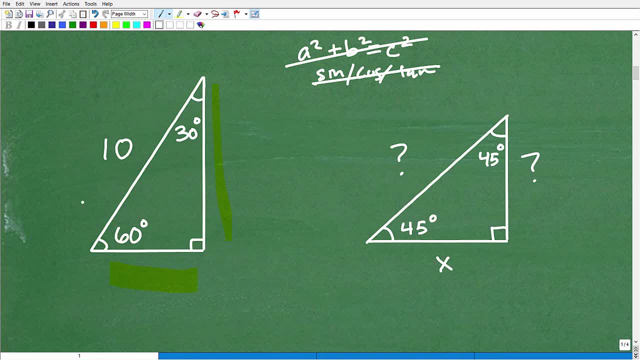 Well, if the hypotenuse is 10, I know the smallest side is going to be half of that. So that's 10 divided by 2, or 5.. I'm like, okay, so now I know this one, I know that this side is going to be whatever. 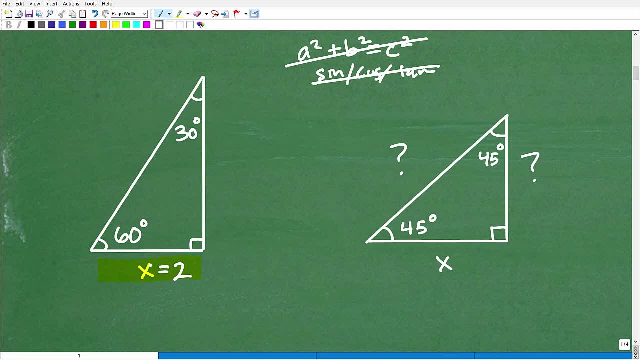 will always be in this proportion. So here is how it goes. all right, If this side is x, the hypotenuse will always be 2x. Okay, So it's double the smallest side. So this is the smallest side. 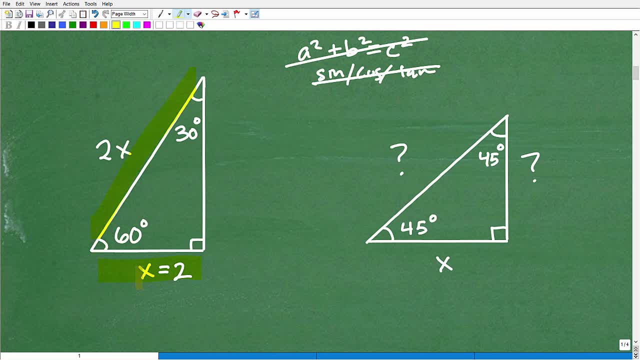 So this hypotenuse, the longest side will be double the smallest side. So that's really easy. That's 2 times 2, or 4.. So you're like, oh wow, that's super easy. 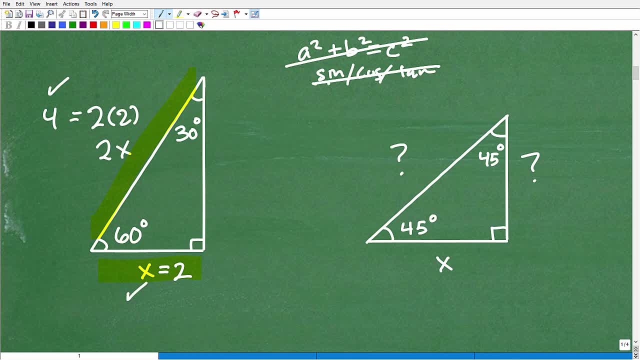 Now I have two lengths. Now, technically, you could now go and use the Pythagorean Theorem, but there's no need to do that. okay, This middle length. okay, not the shortest, not the longest, but this middle one. 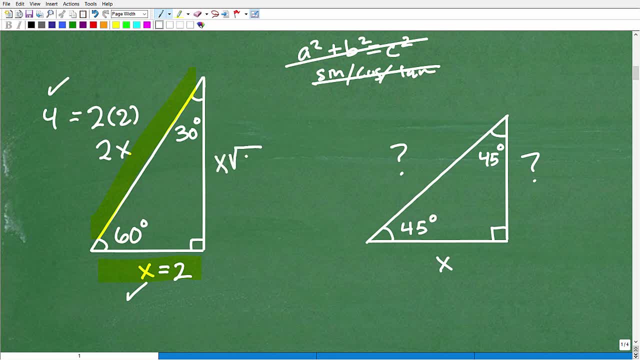 this one right here, This middle length right here is going to be x times the square root of 3.. So, whatever this value is here, this is 2 in this particular problem. So we just take that 2, and we multiply it by the square root of 3, and that's what this is. 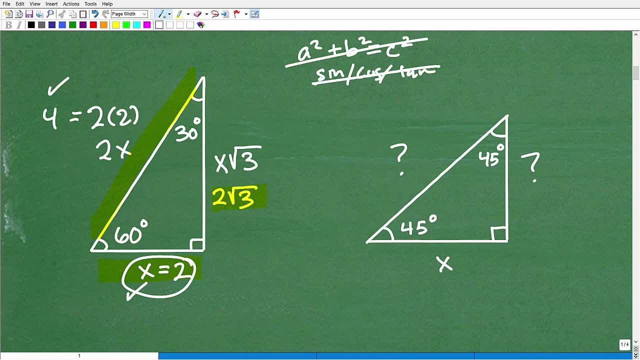 I mean easy as 1,, 2,, 3.. Now there's a lot more sophisticated kind of problems that you could do. I could give you this length of a 30-60-90, and then you would have to go and determine that. 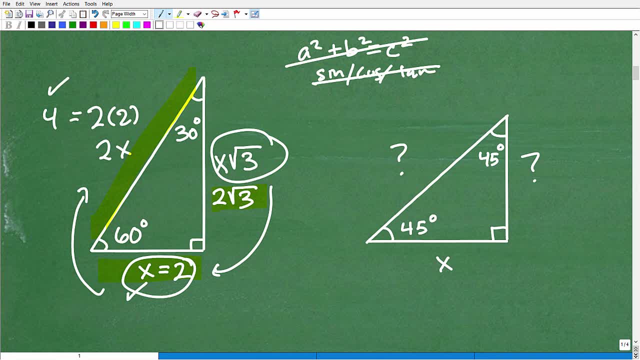 and then you could determine this, Or I could give you the hypotenuse. Actually, this is the hypotenuse. Actually, this is the hypotenuse. Let's do another quick problem here and let's see if you can remember all of this. 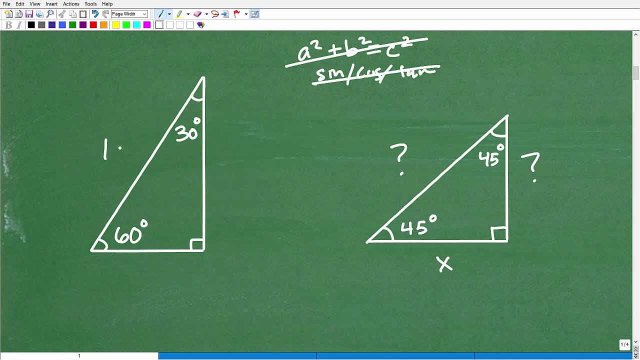 and we'll kind of reverse engineer the solution. So let's say this is 10,. all right, I give you this problem and I want you to know, I want you to go ahead and figure out what these sides are. So how could I approach that? 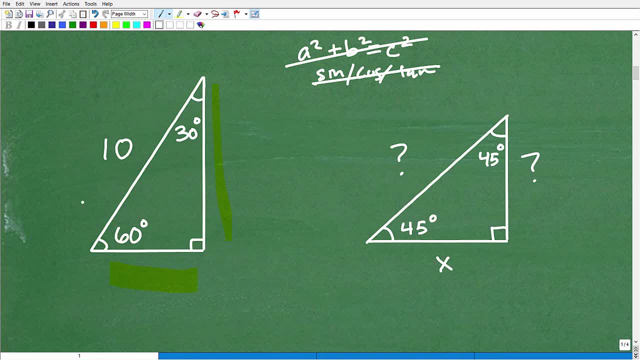 Well, if the hypotenuse is 10, I know the smallest side is going to be half of that. So that's 10 divided by 2, or 5.. I'm like, okay, so now I know this one, I know that this side is going to be whatever. 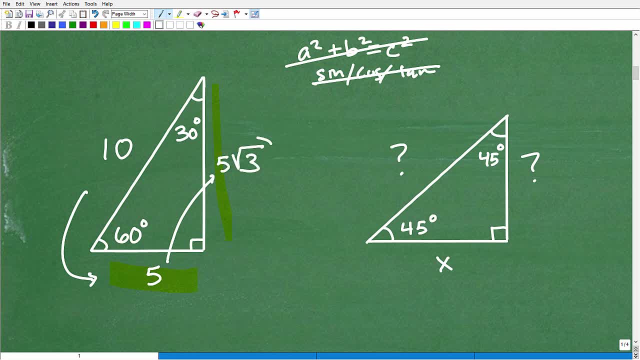 this side is 5 times the square root of 3, and I'm done 1,, 2, and 3, okay, So that's the beauty of knowing about these special right triangles. These come up all the time, but let me when I tell you you need to know how to deal with. 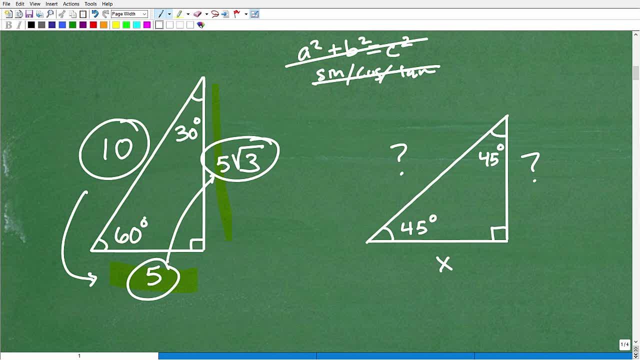 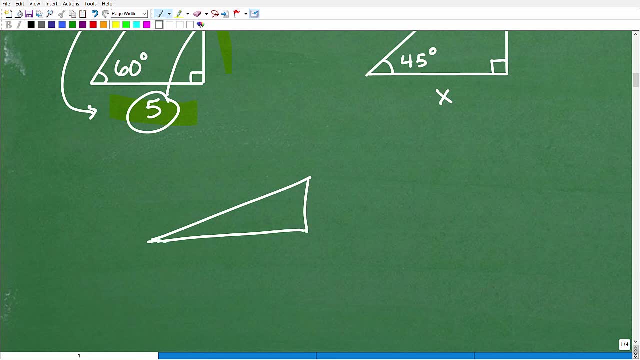 30-60-90 right triangles And, by the way, you may not see them. you know, like this, You might see it kind of this way. You might see it like: so okay, All right, I'm just kind of sketching. 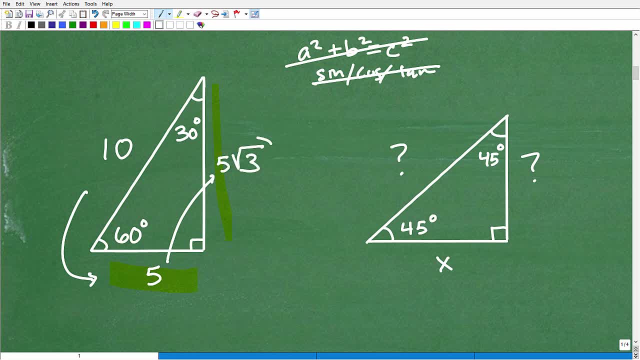 this side is 5 times the square root of 3, and I'm done 1,, 2, and 3, okay, So that's the beauty of knowing about these special right triangles. These come up all the time, but let me when I tell you you need to know how to deal with. 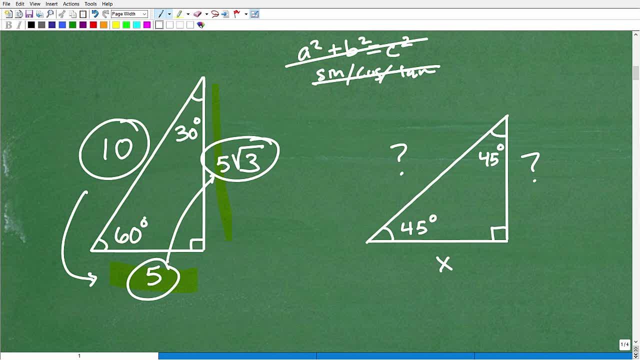 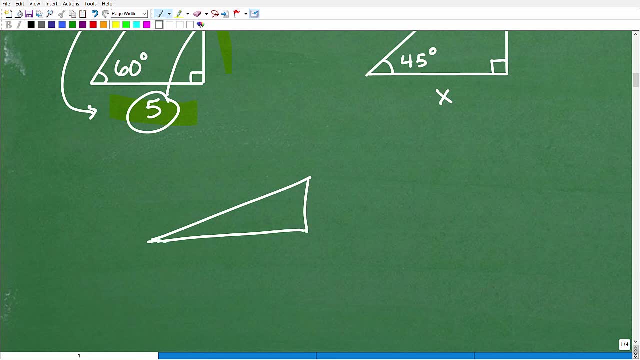 30-60-90 right triangles And, by the way, you may not see them. you know, like this, You might see it kind of this way. You might see it like: so okay, All right, I'm just kind of sketching. 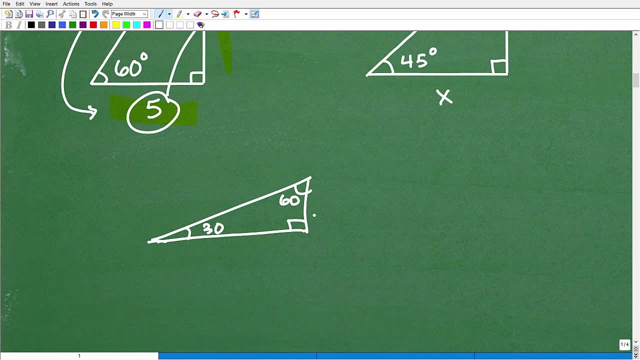 Does this be our 30?? And this would be. This is our 60, and this is our 90.. So, in that case, this is x, This would be 2x and this is x times the square root of 3.. 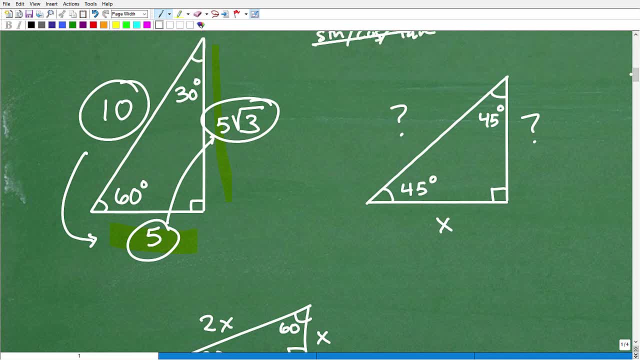 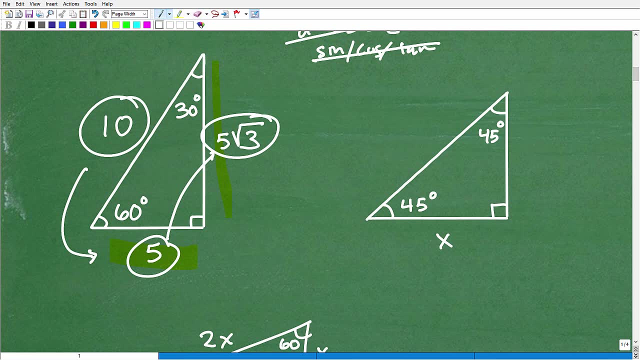 Okay. so now let's go to our 45-45-90 situation. This is quite easy- this one here- because when you have a 45-45, whatever- this side is right. here this is like a square and it's diagonal. 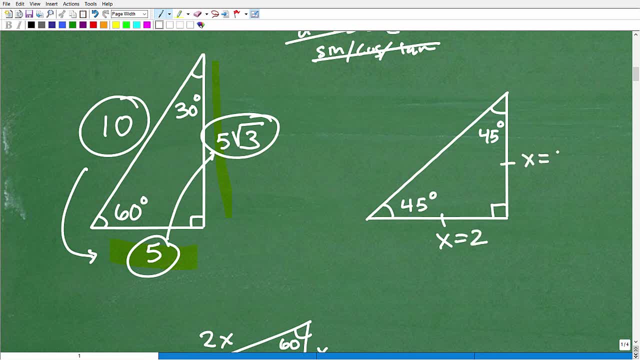 This side is also x, So if this is 2, this side is also 2.. I mean, it's pretty easy, right? So now here you would say: okay, well, I have enough information to go ahead and figure. 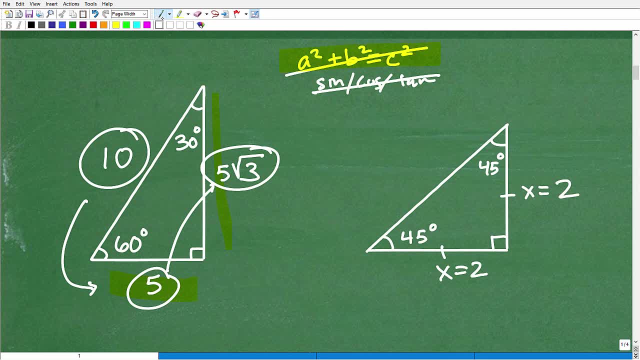 out the hypotenuse. I could use the Pythagorean theorem. Yes, you could, but if you have a 45-45, all you need to know is that this side will be x times the square root of 2, all right. 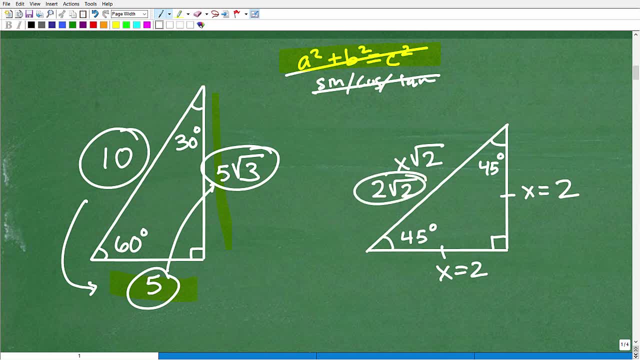 So that would be 2 square root of 2 is our answer. You know you don't want to go ahead and do this. 2 squared plus 2 squared is equal to c squared, So this is 4.. 4 plus 4, right. 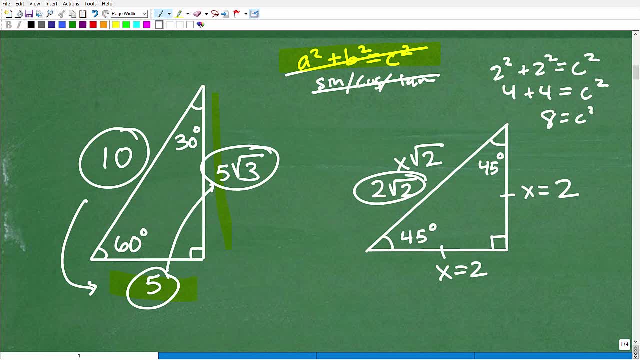 That's c squared and that would be 8 equals c squared. We take the square root of both sides, so I get c is equal to the square root of 8.. Let's see how your algebra is. All right, we can go down here. take the square root of 8.. 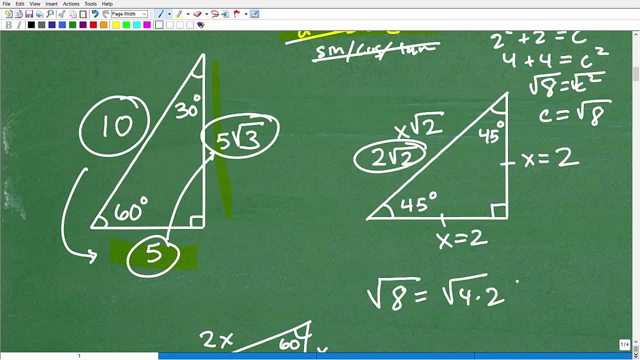 That factors as a square root of 4 times 2,, or a square root of 4 times a square root of 2, or 2 square root of 2.. Look at all that work. If I just knew the rule, And I take this side and a 45-45, and multiply it by square root of 2, I just write the answer. 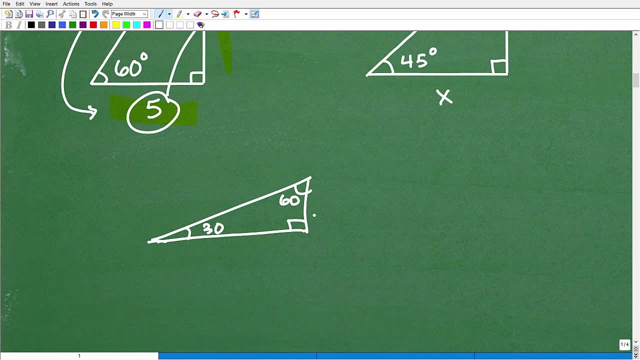 Does this be our 30?? And this would be. This is our 60, and this is our 90.. So, in that case, this is x, This would be 2x and this is x times the square root of 3.. 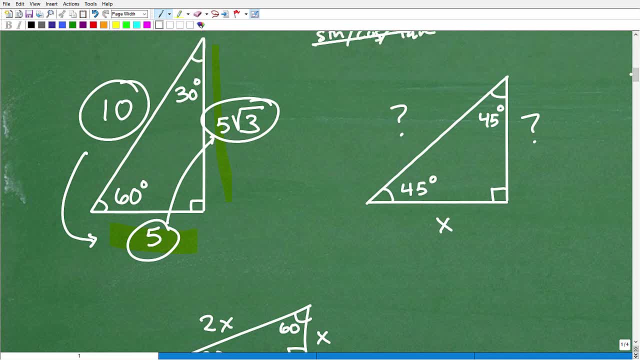 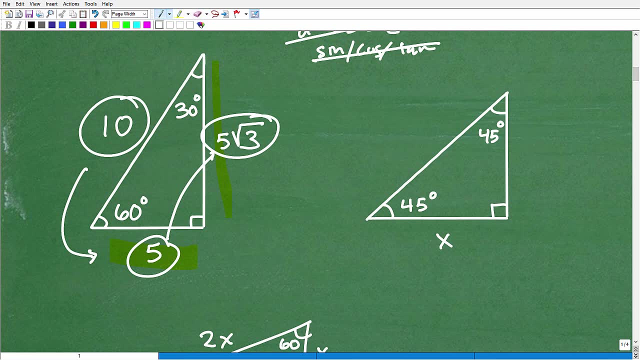 Okay. so now let's go to our 45-45-90 situation. This is quite easy- this one here- because when you have a 45-45, whatever- this side is right. here this is like a square and it's diagonal. 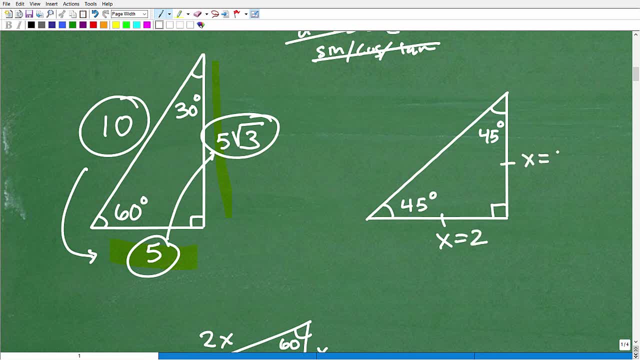 This side is also x, So if this is 2, this side is also 2.. I mean, it's pretty easy, right? So now here you would say: okay, well, I have enough information to go ahead and figure. 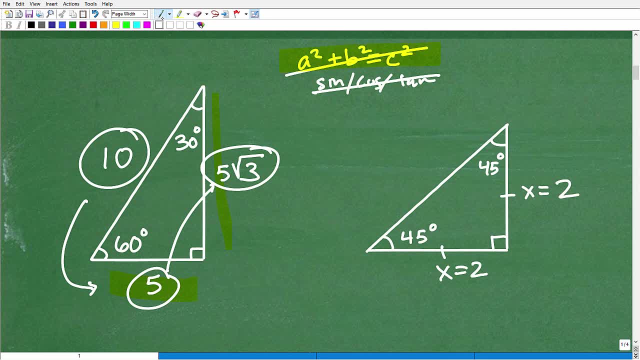 out the hypotenuse. I could use the Pythagorean theorem. Yes, you could, but if you have a 45-45, all you need to know is that this side will be x times the square root of 2, all right. 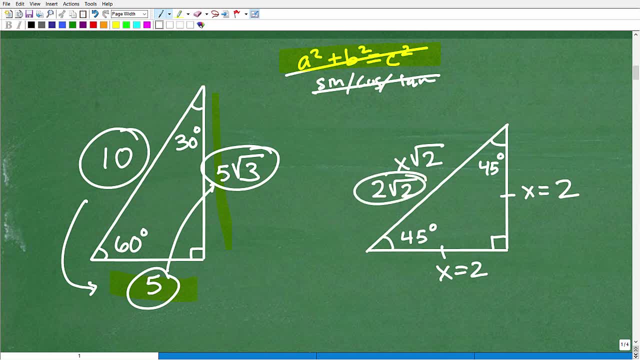 So that would be 2 square root of 2 is our answer. You know you don't want to go ahead and do this. 2 squared plus 2 squared is equal to c squared, So this is 4.. 4 plus 4, right. 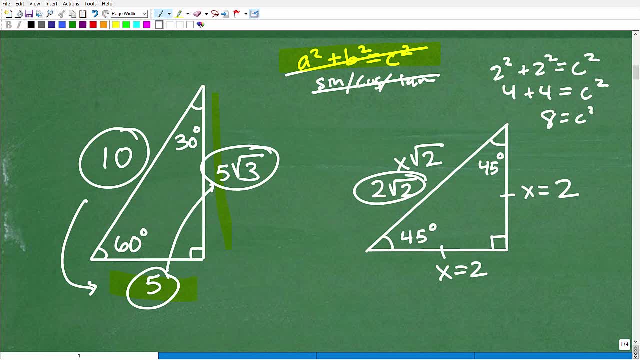 That's c squared and that would be 8 equals c squared. We take the square root of both sides, so I get c is equal to the square root of 8.. Let's see how your algebra is. All right, we can go down here. take the square root of 8.. 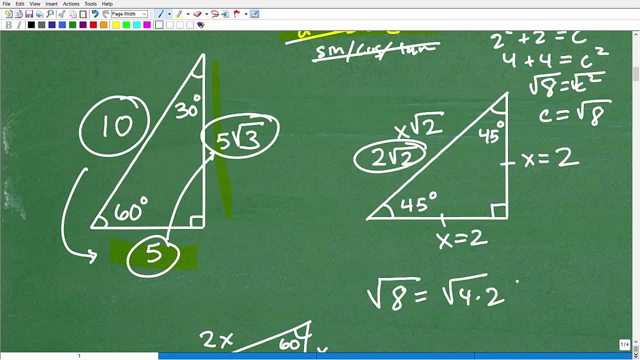 That factors as a square root of 4 times 2,, or a square root of 4 times a square root of 2, or 2 square root of 2.. Look at all that work. If I just knew the rule, And I take this side and a 45-45, and multiply it by square root of 2, I just write the answer. 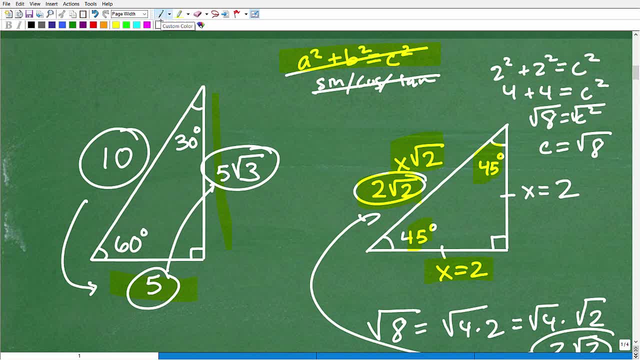 okay, So you're going to encounter again 45-45, 90s, 30-60, 90s. This is going to be something you will see, okay, You'll see it on some exam and you certainly need to know this in geometry, okay. 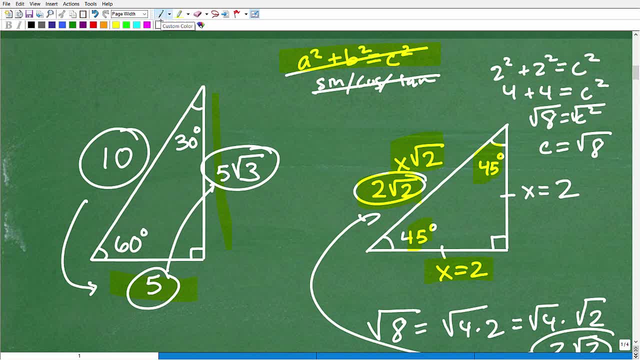 okay, So you're going to encounter again 45-45, 90s, 30-60, 90s. This is going to be something you will see, okay, You'll see it on some exam and you certainly need to know this in geometry, okay. 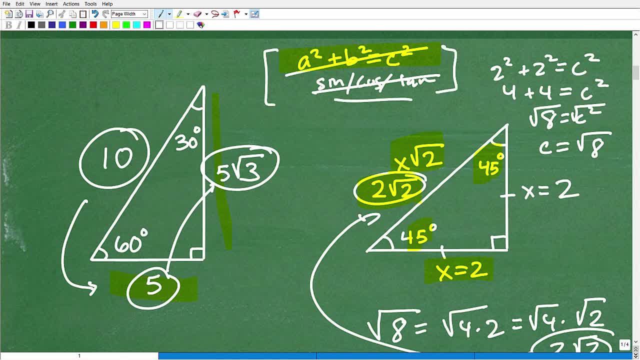 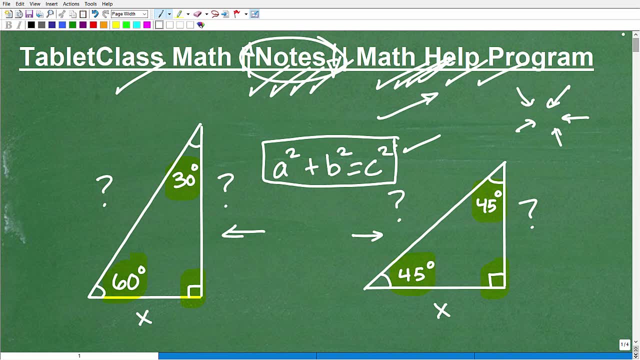 But you know not to minimize the Pythagorean theorem and basic right triangle trigonometry. You've got to know that as well. But again, What we're dealing with here is special right triangles. You've got to know special right triangles. 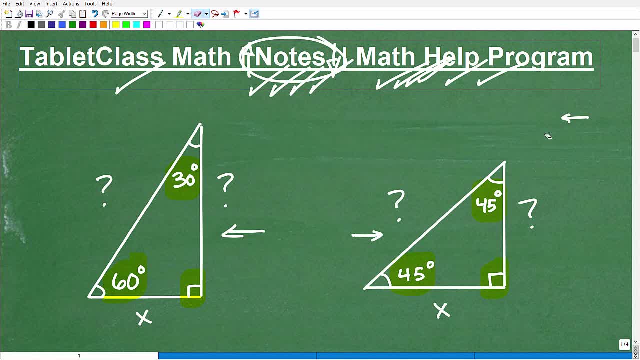 And hopefully okay. this video was a good introduction to them and a good review. Like anything, you'll want to practice more sophisticated problems. I can make more challenging problems, But if you just keep those proportions in mind, you're going to do just fine. 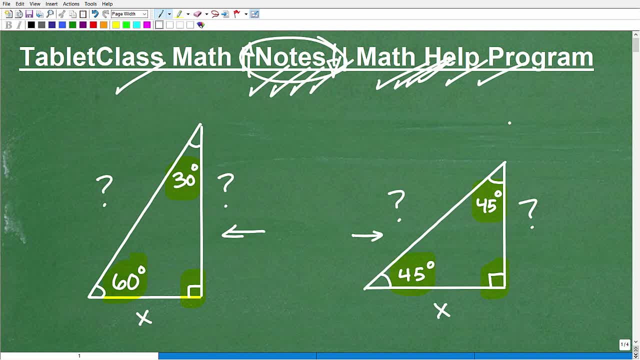 Okay. so if this video helped you out in some way, if you enjoyed this video, if you were like, yeah, that was worth watching, I learned something, then please consider smashing that like button. That always helps me out And also, hopefully, you'll consider subscribing. 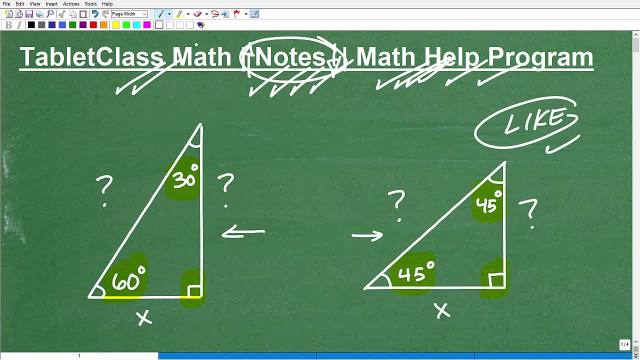 I've been on YouTube for a long time, have hundreds and hundreds of videos organizing basic to advanced mathematics. It's a great platform for someone like myself who's obsessed with teaching math in a clear and understandable way. My job, you know, my passion, is to get you to you know, understand math. 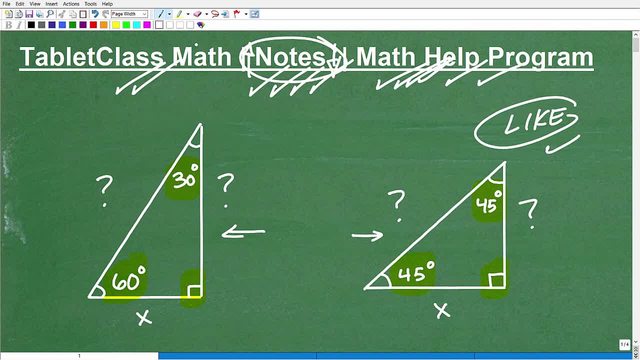 You know if you're struggling with math. you know, typically people don't like math because they're frustrated with it. They're having a difficult time learning. If you learn things, all right and it doesn't have to be like torture, you know. 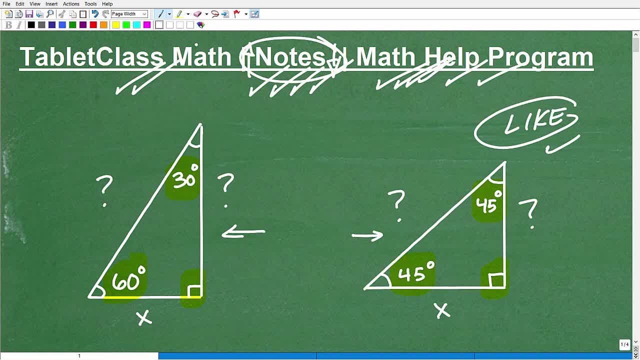 you're like: okay, I get this. If you have to study this topic, okay, let's try to make it. you know in a way, that's not terrible. you know in a way that you're okay, I'm learning. 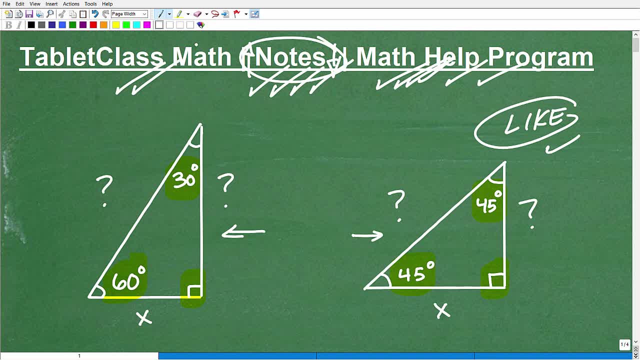 I can do this. Let me learn the math that I need to learn to get me to my goals. Okay, so that's how I kind of view things. Not everyone's going to want to be a mathematician engineer. I get that. 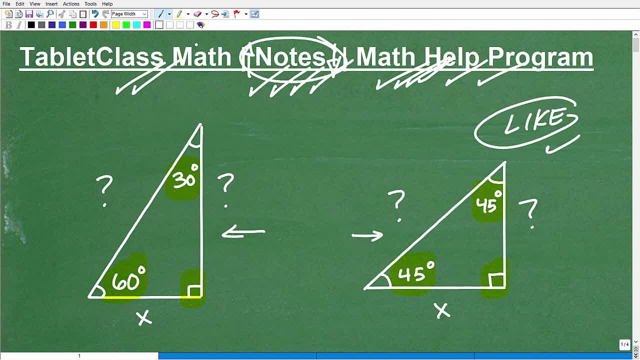 But guess what Many of you, if you're studying, if you're looking at this video, you need to learn math to get where you want to go, whatever goal, Maybe it's passing one of those tests I was talking about, or placing into college. 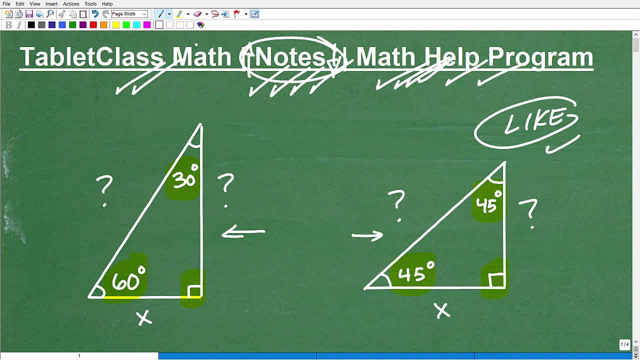 or whatever the case might be, or just getting a good grade in your current math class. right, You got to learn mathematics to get it. There's only one way to learn, and that is to you know, have a good attitude and work hard. 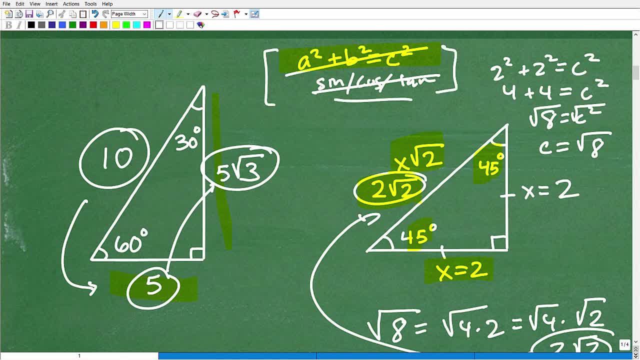 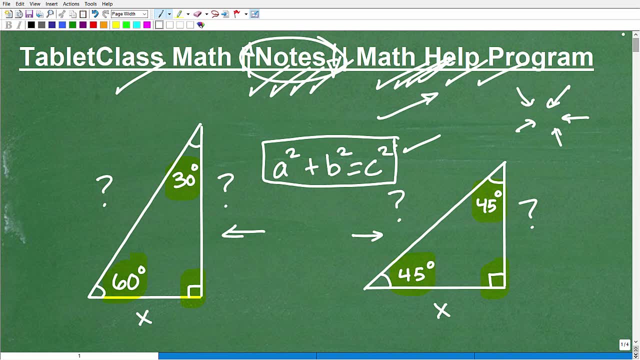 But you know not to minimize the Pythagorean theorem and basic right triangle trigonometry. You've got to know that as well. But again, What we're dealing with here is special right triangles. You've got to know special right triangles. 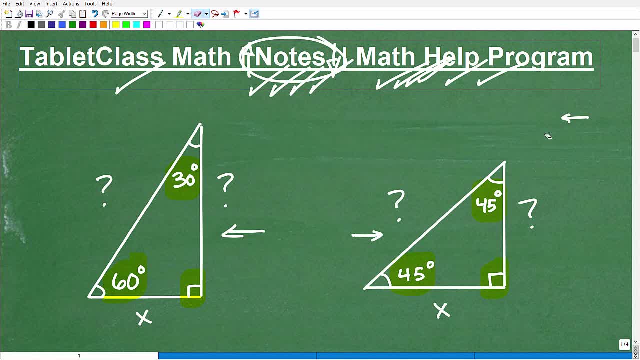 And hopefully okay. this video was a good introduction to them and a good review. Like anything, you'll want to practice more sophisticated problems. I can make more challenging problems, But if you just keep those proportions in mind, you're going to do just fine. 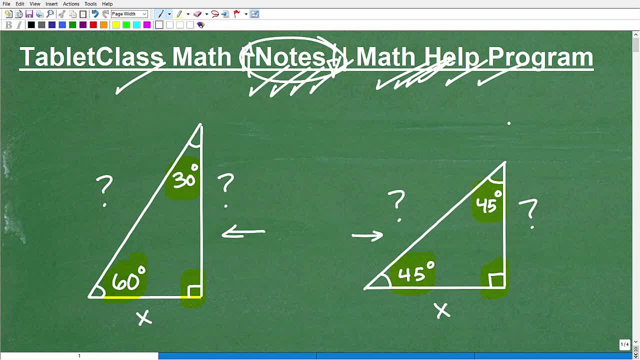 Okay. so if this video helped you out in some way, if you enjoyed this video, if you were like, yeah, that was worth watching, I learned something, then please consider smashing that like button. That always helps me out And also, hopefully, you'll consider subscribing. 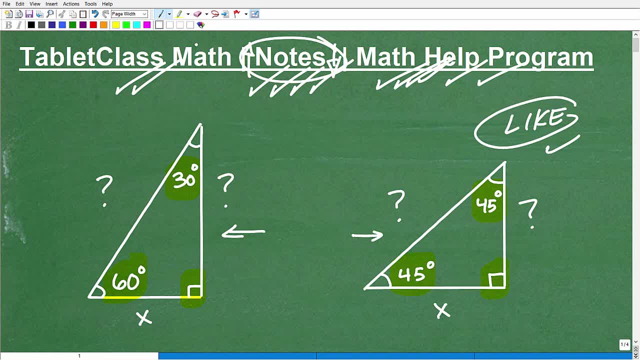 I've been on YouTube for a long time, have hundreds and hundreds of videos organizing basic to advanced mathematics. It's a great platform for someone like myself who's obsessed with teaching math in a clear and understandable way. My job, you know, my passion, is to get you to you know, understand math. 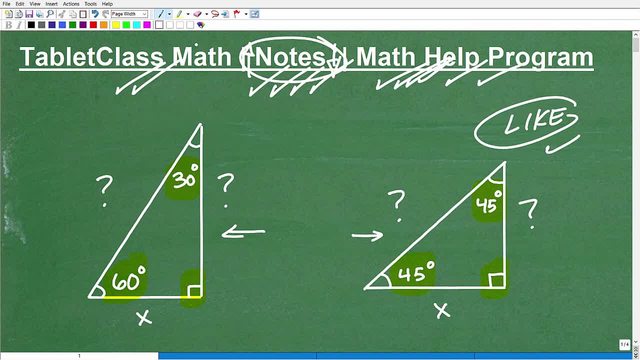 You know if you're struggling with math. you know, typically people don't like math because they're frustrated with it. They're having a difficult time learning. If you learn things, all right and it doesn't have to be like torture, you know. 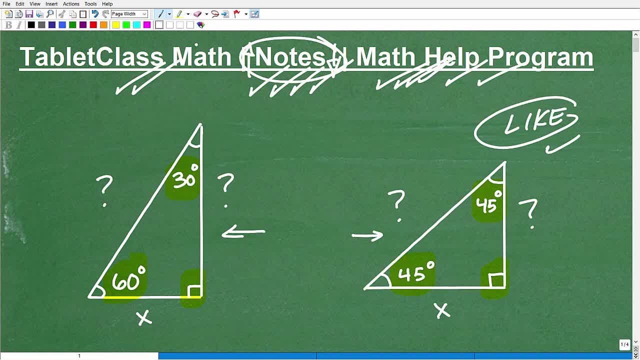 you're like: okay, I get this. If you have to study this topic, okay, let's try to make it. you know in a way, that's not terrible. you know in a way that you're okay, I'm learning. 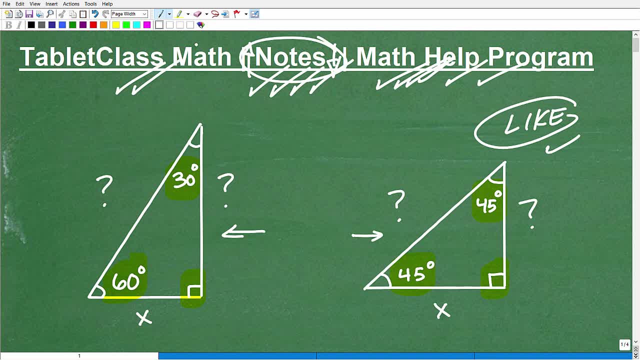 I can do this. Let me learn the math that I need to learn to get me to my goals. Okay, so that's how I kind of view things. Not everyone's going to want to be a mathematician engineer. I get that. 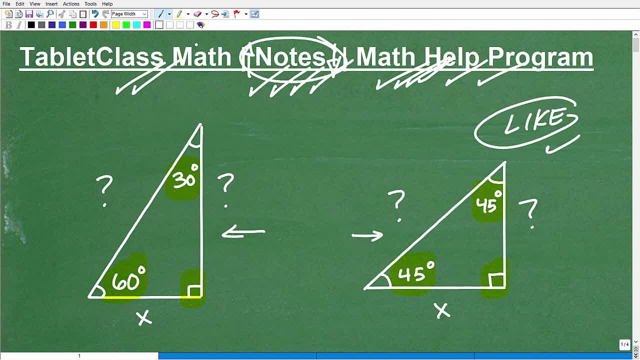 But guess what Many of you, if you're studying, if you're looking at this video, you need to learn math to get where you want to go, whatever goal, Maybe it's passing one of those tests I was talking about, or placing into college. 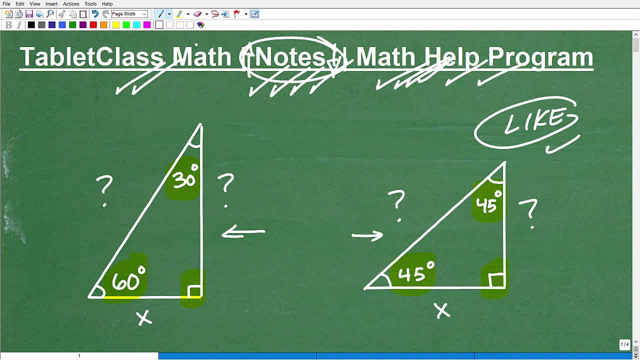 or whatever the case might be, or just getting a good grade in your current math class. right, You got to learn mathematics to get it. There's only one way to learn, and that is to you know, have a good attitude and work hard. 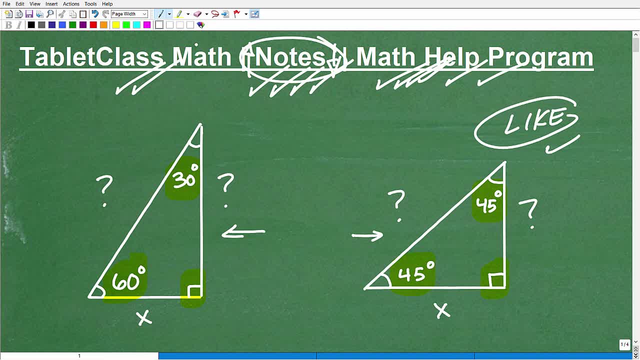 Okay, so again, if you wanted more additional information on all this stuff, just check out my videos in my various playlists on my channel. But you know my best work will always be in my Math Help program. Okay, so, with that being said, I definitely wish you all the best in your mathematics adventures. Thank you for your time and have a great day.